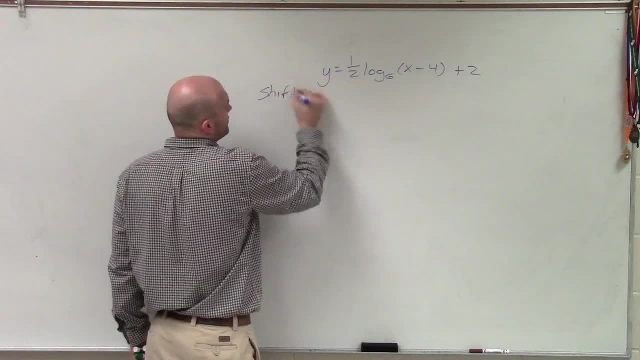 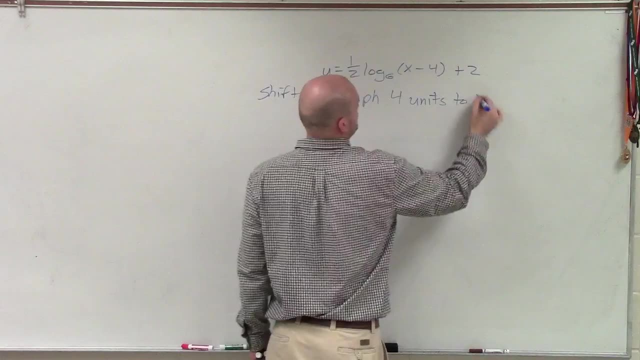 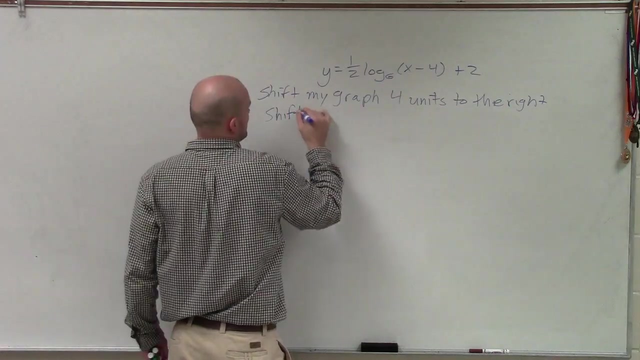 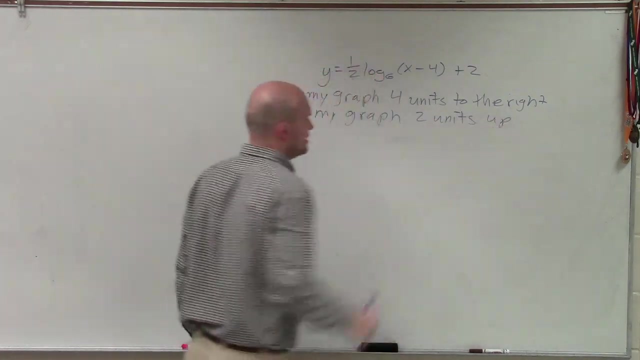 graph. Well, the x minus 4 is going to tell me I'm going to shift my graph 4 units to the right, And then the plus 2 is going to tell me to shift my graph 2 units up. So what I need to do is: what am I shifting 4 units to the right and 2 units up from? So to do? 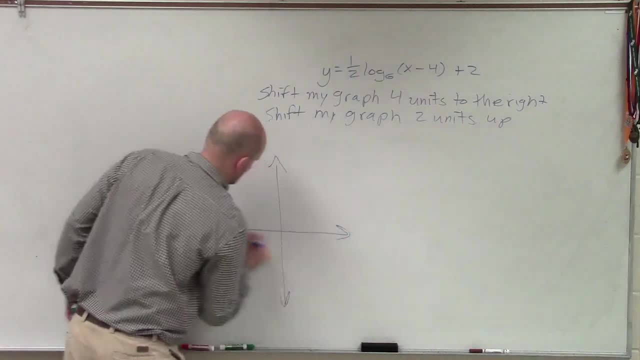 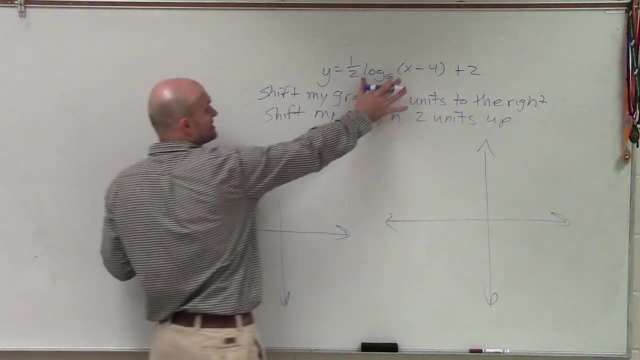 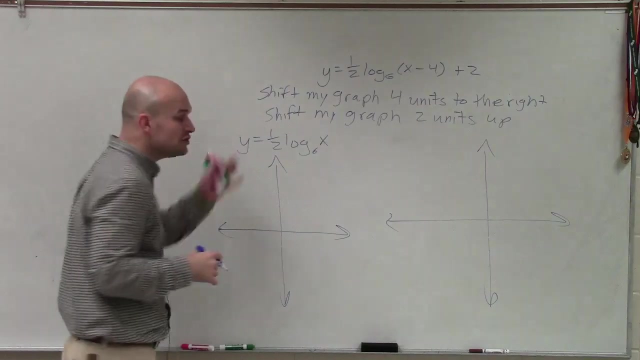 that we want to graph our parent function And we also. then here is going to be our final graph, So our parent function, And we're just going to take this without the transformations. It would be: y equals 1 half log base 6 of x. Now you can do it without the 1 half and then just take those. 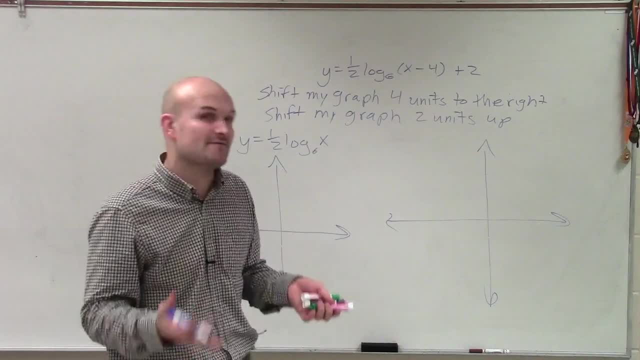 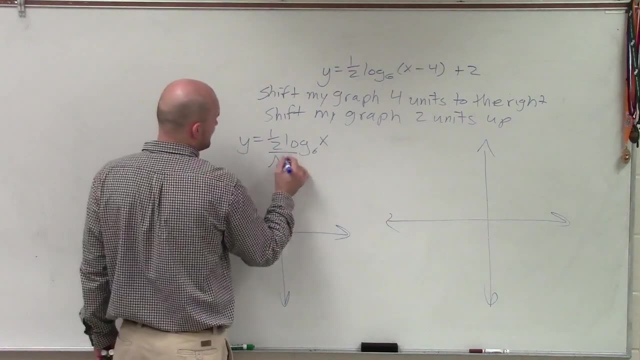 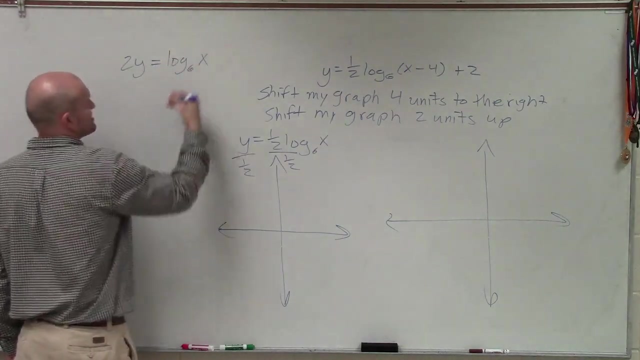 points and multiply them by your x values by 1 half, if you want to, But I like to leave this in here because when I rewrite this in exponential form, what I like to do is divide by 1 half. So therefore, it's 2y equals log base 6 of x. Then, when I rewrite this in exponential 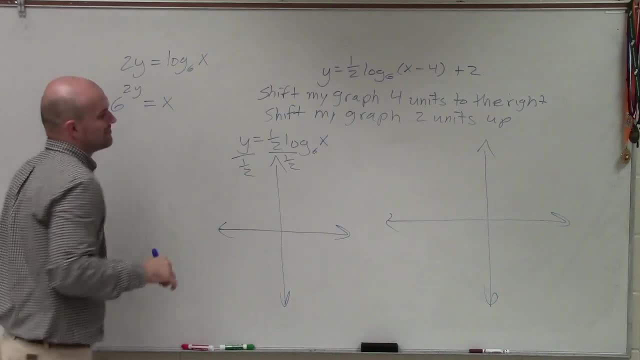 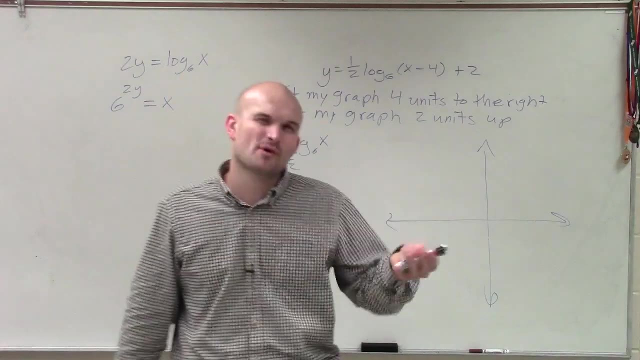 form I have: 6 raised to the 2y equals x, And again you can graph the parent function without the 1 half and then just multiply each of those points, But then again you're just doing more and more dilations, which I like to kind of get it out of the way. So 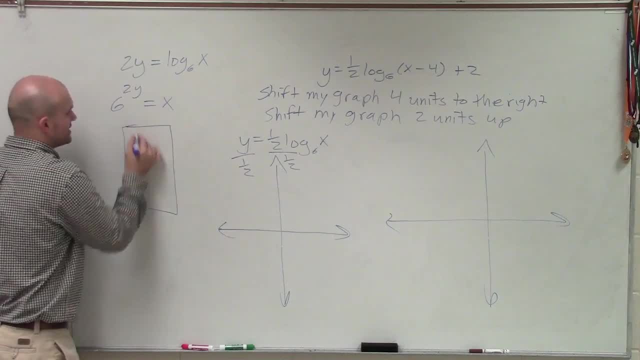 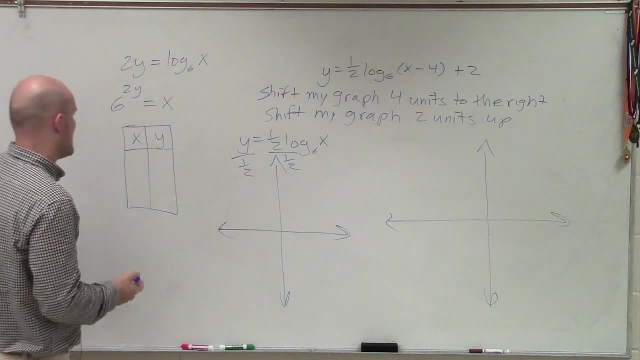 now what I want to do is create a table of values for this graph, So I have my x and my y's And a lot of times again. what I like to do when I'm choosing my x values is: I want to choose when is x going to equal 1? And when is x going to equal the base And when? 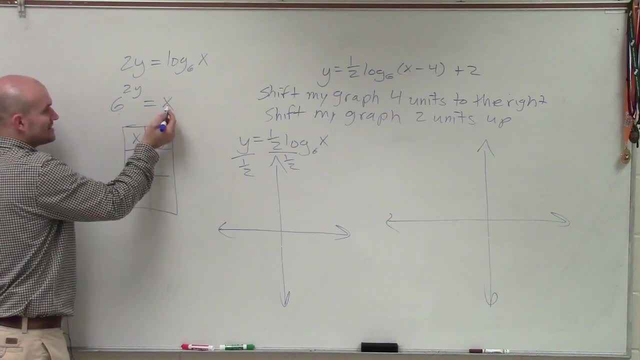 is x going to equal the base, And that's what I want to do, So I'm going to do this. So x is going to equal the base of 6.. So x equals 1, obviously when 6 is raised to a power of 0. 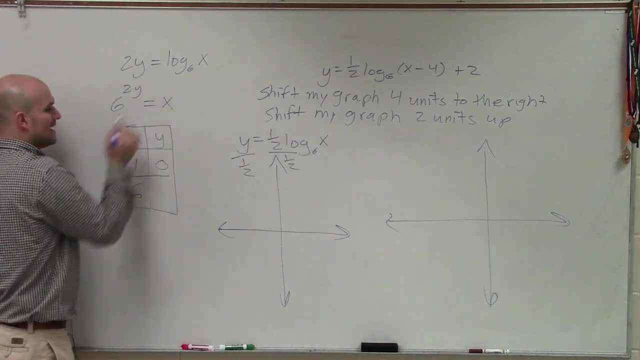 6 is going to be raised to a power of 0 when y equals 0. Then I need to look at: well, when is x going to equal 6?? That means this is going to be raised to a power of 1.. 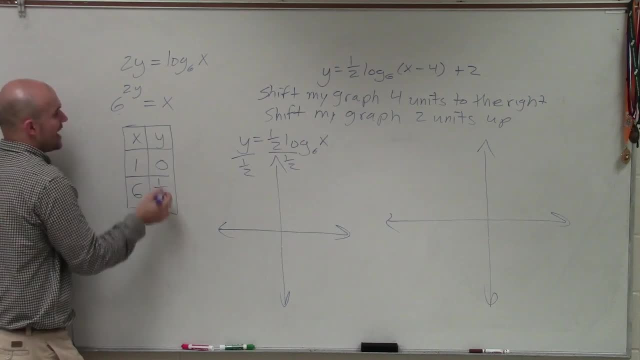 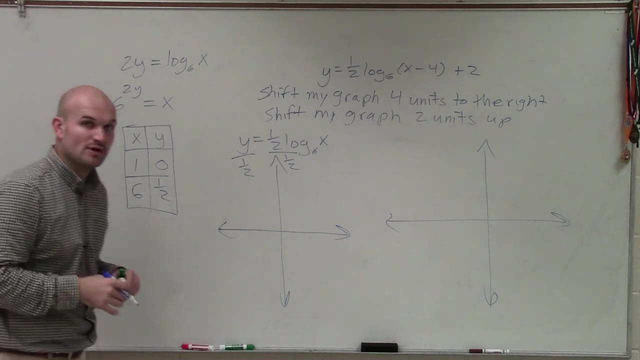 Well, 2 times 1 is going to leave me with 1 half. So when y equals 1 half, 1 half times 2 is 1.. 6 raised to the first power is just going to equal 6.. So now I have these two coordinate points. 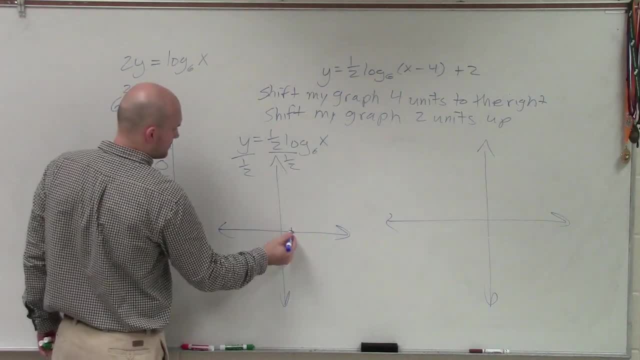 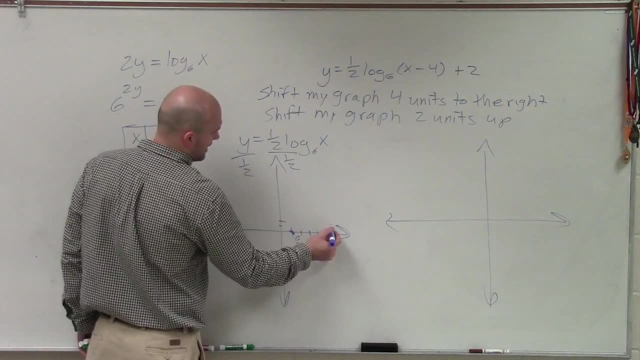 that I'm going to want to graph 1 comma 0, and then 6 comma 1 half. So 1,, 2,, 3,, 4,, 5, 6, up 1 half. So, therefore, my graph is going to look something like this: 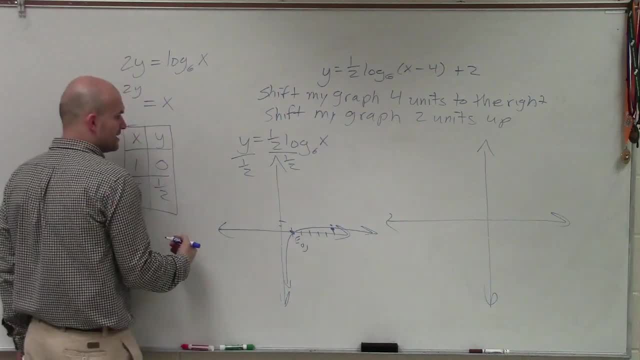 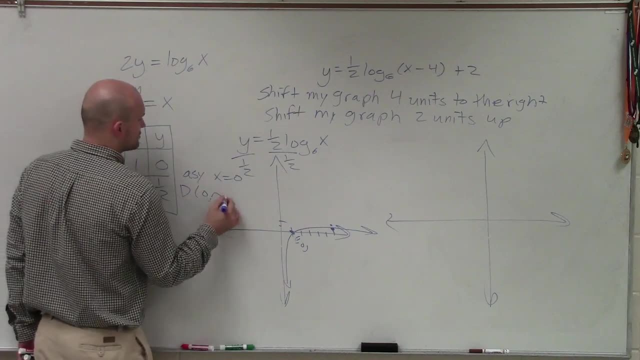 It's going to have a very, very sharp turn. When, looking at my graph, I know that my asymptote is at: x equals 0. My domain is from 0 to infinity And my range is from negative infinity to infinity. That's just the basis of understanding. 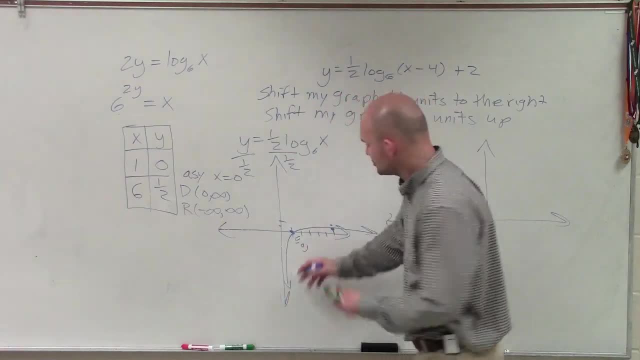 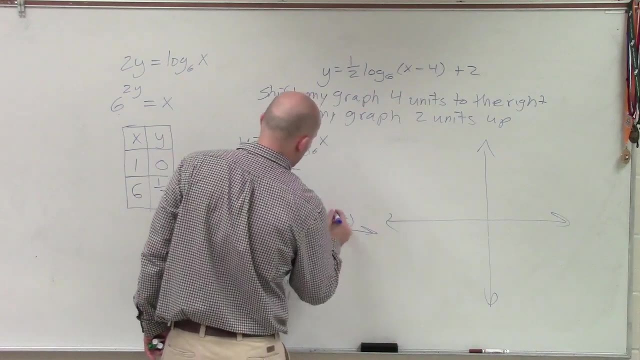 what the parent graph is going to be looking like. But just notice, on this graph it has a very, very sharp turn. But the main important thing, what I want to do, is take these points, And what I'm going to do now is now transfer these four units. 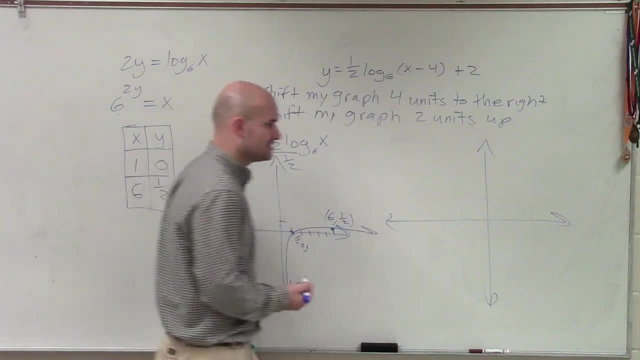 to the right. So instead of dealing with the point 1 comma 0,, I'm now going to deal with the point 5, comma 0.. 1,, 2,, 3,, 4,, 5.. And instead of dealing with the point 6, comma 1, half. 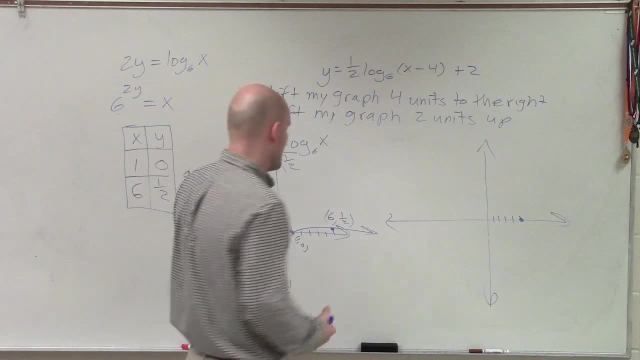 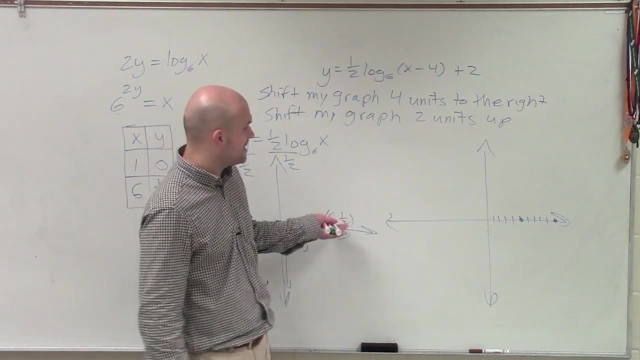 I'm now going to deal with a point 10 comma 1 half. So 5,, 6,, 7.. 8,, 9,, 10.. But now I'm not going to be shifting them now. or 6 comma 1 half. 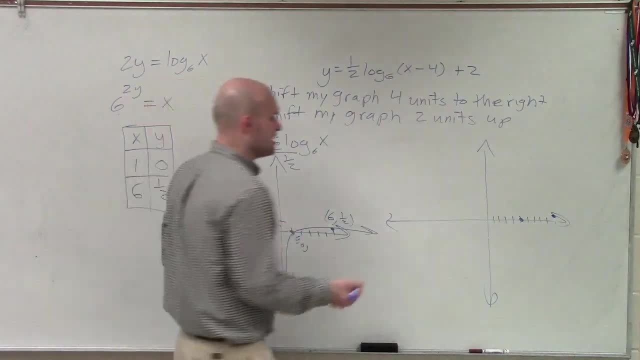 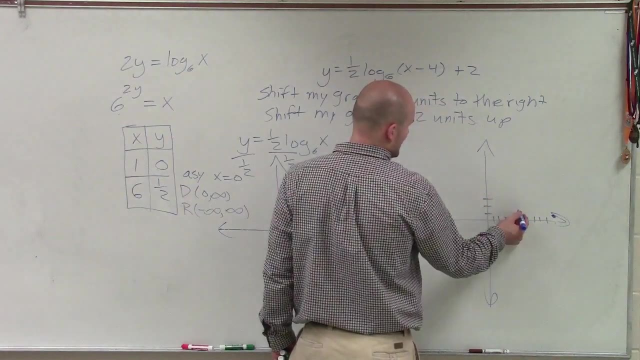 But now what's going to happen is I'm going to shift this graph also two units up. So let's say: here's 1, here's 2.. So, therefore, and there will be 3.. So up 2 would be now instead of at 0, now it's up to 2.. 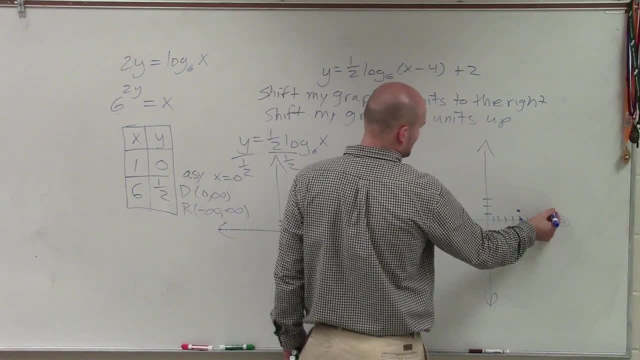 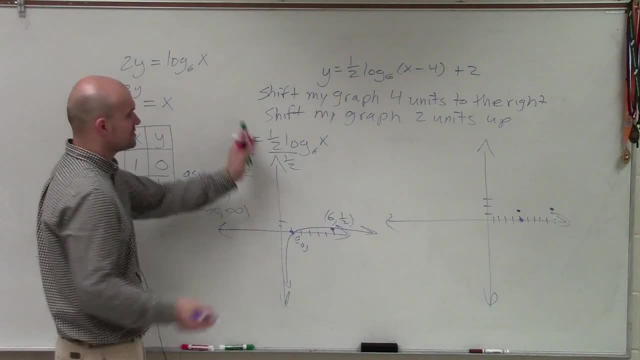 And it started at 1 half. It's now going to be at 2 and 1 half. All right, now the next thing. what I always like to do is draw the asymptote first. My asymptote was originally at x equals 0.. 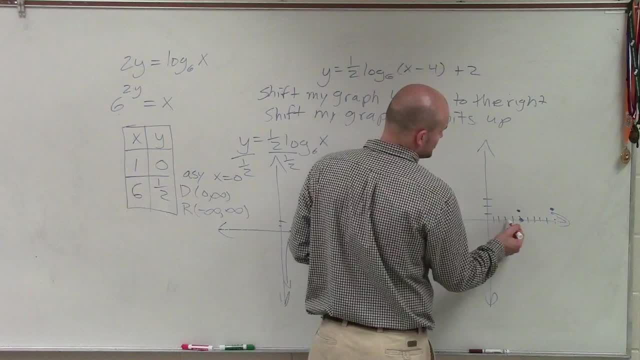 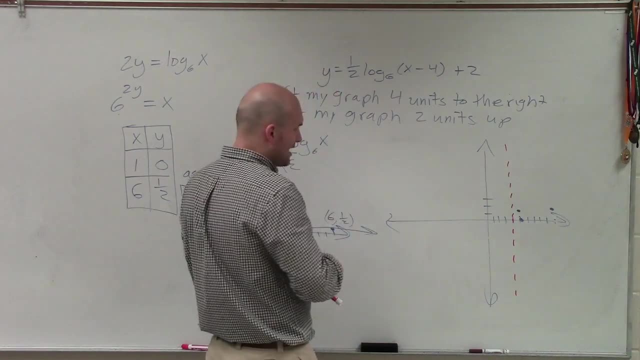 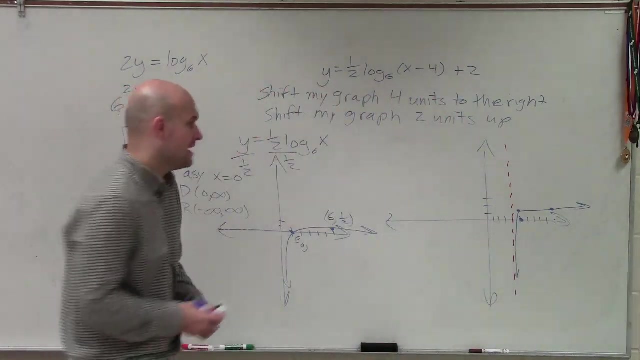 That asymptote has now been moved to: x equals 4.. 1,, 2,, 3,, 4.. Because the graph was shifted four units to the right. All right, so now I can graph this And you can see it has this very, very sharp turn. 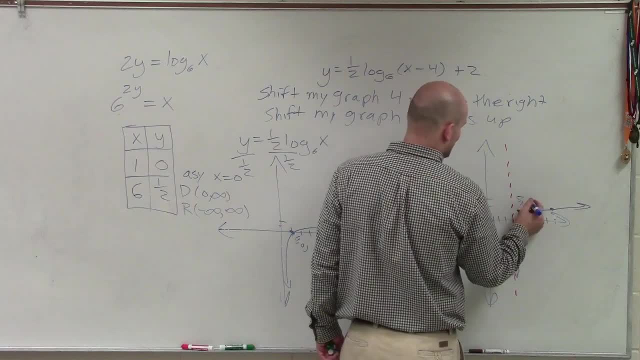 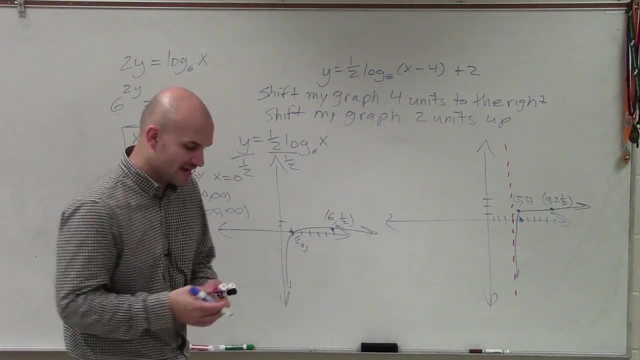 And my two points again are 5 comma 2.. And now 10 comma 2 and 1 half. All right, But now we need to understand that our domain and range and asymptote have changed. Our asymptote is no longer at x equals 0..